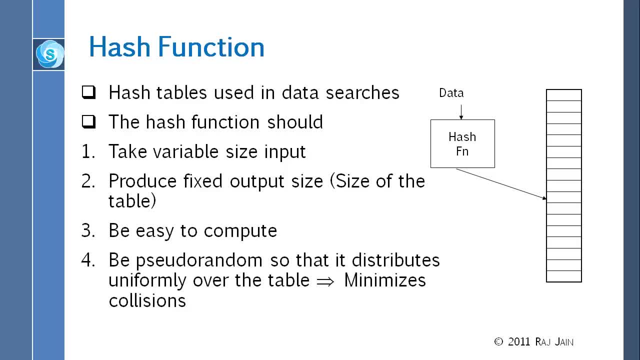 When you want to look it up, instead of searching through the whole table, you hash it and go and look up right there. If you want to look it up instead of searching through the whole table, you hash it and go and look up right there. 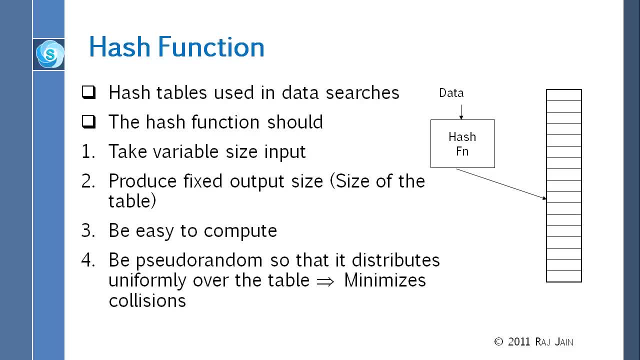 If there's a clash then you look up at the next entry, and so on and so forth. So that's the fastest way to do search and entry. If you have a large table, the larger the table, the better decision to do hashing. 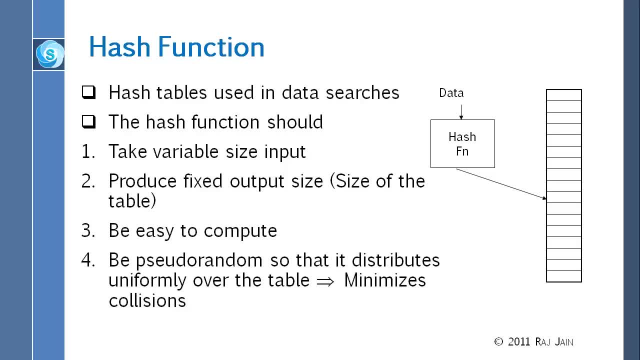 Because if you do linear search, it is log n, If you do binary search, it is log n, And binary search requires sorting and everything else. With hash, you don't need sorting, you don't need searching. Is that clear? Everybody has used hash in one way or the other. 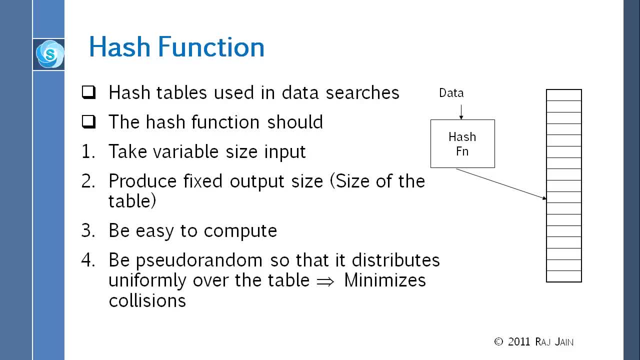 Yes. If not, I understand how to use it And generally with hash functions, what we do is we make the table much larger, the space, so that there are lots of empty space. So the collisions are very few. So that's normal hash function. 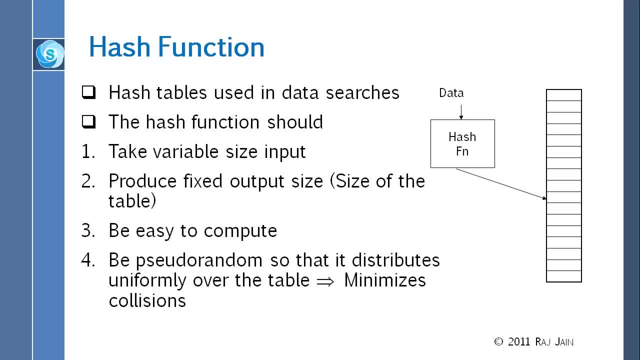 And in networks we use the hash function, particularly when we have to search through. Remember, the Ethernet MAC addresses are basically not in any order, They're just random. Basically, you could have any address anywhere. It's universally unique. So the only way you can find out whether the MAC address in your table is to just search through a big table. 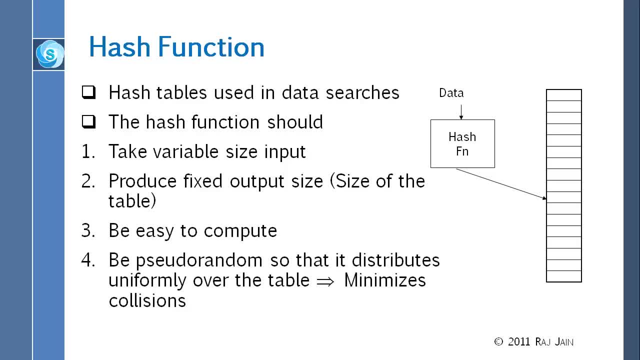 If you see a packet for a particular MAC address, source destination, whatever it is, you have to look it up, The only way to do that. in that respect, I have done a study of hash functions. I have a paper on what is the best hash function. 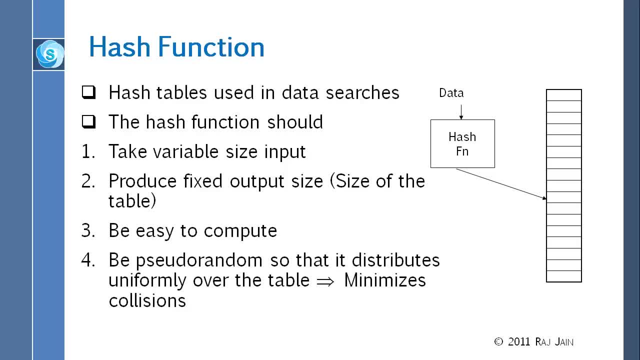 But that was done for this kind of purpose. Looking up in the MAC addresses And the best hash function, the conclusion of that study was: the best hash function is the Ethernet CRC. What that means is you could take any MAC address which is 48-bit long. do the Ethernet CRC on it. 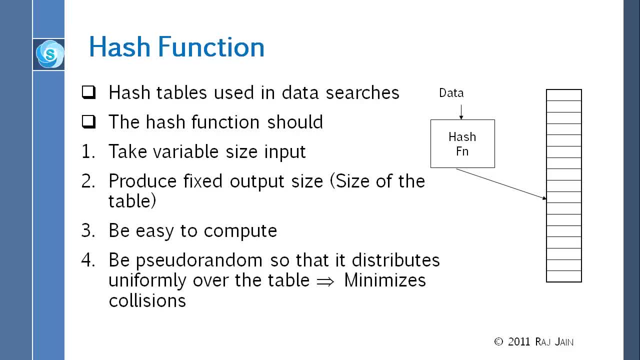 You will get a 32-bit And you can take any number of bits from there to make up your table. That's a very good hash function And clearly that was the best in all the tests we did. All right. So hash functions should be: should take variable size input, put a fixed size output. should be easy to compute. 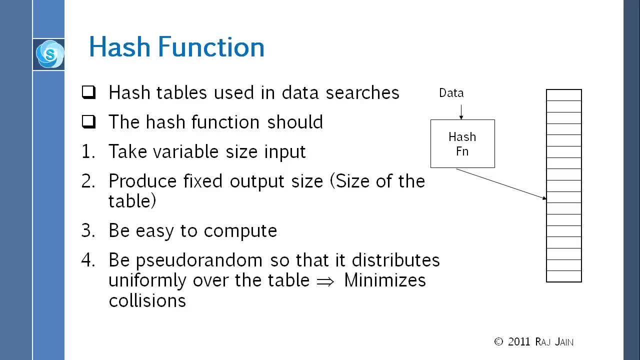 and should be pseudo-random so that it distributes equally over the table and minimizes the collision. So there are lots of functions for hash And, as I said, CRC checksums are you know best, All right, But they are not very good for cryptographic purposes. 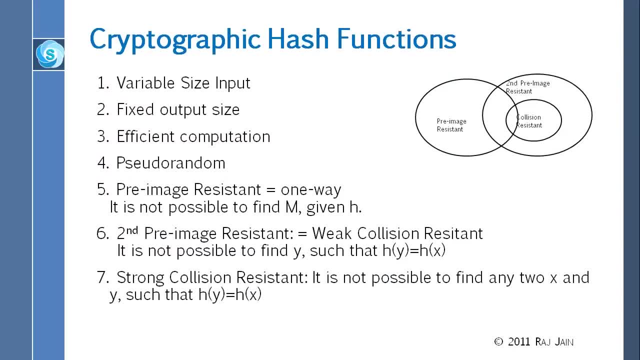 For cryptography you need, if nothing else, you need- one-way property, such that if somebody gave you the hash, you cannot find the original key, Because- and then second thing is: so there are many properties. So first let's start with the first four properties, which are properties of the hash functions. 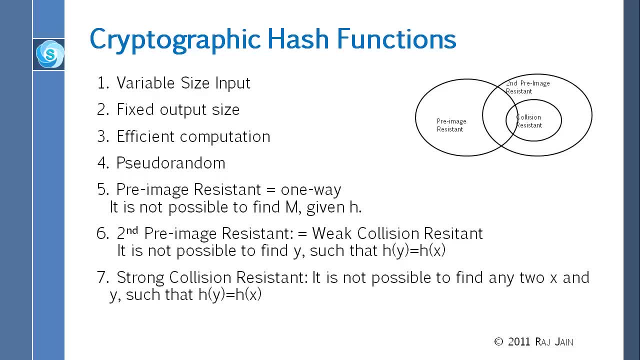 They take variable size input output. the fixed size output are easy to compute and they are pseudo-random, So this is a normal hash function. But the three more things are added for cryptography, And the first thing is it should be one-way. 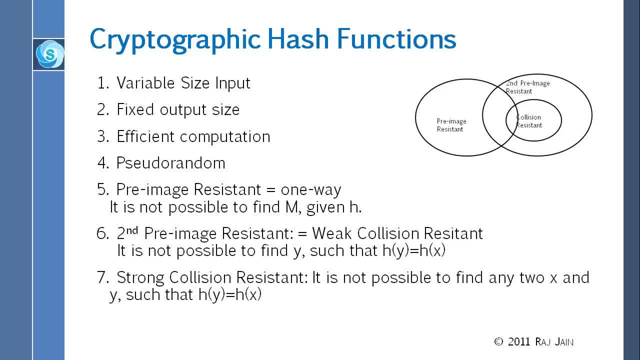 So if, given somebody gave you H, you cannot find M. Given M, it is very easy to compute H. It's one-way, So this is called the technical name for this is pre-image resistant, So before you got the hash you could not find out what the number was. 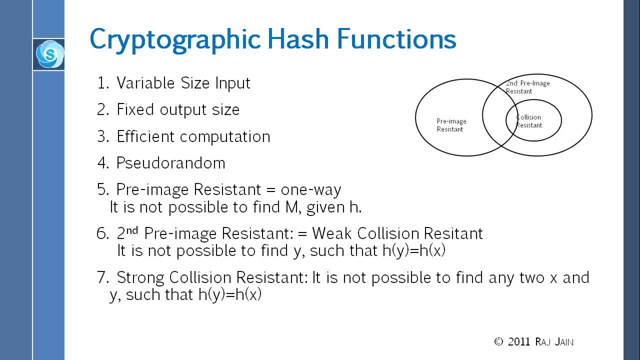 Pre-image resistant. Second property is that, given not only that you cannot find M, but then the second property is that you could not find another Y which has to the same value. So that is called second pre-image resistant, which means that you cannot create collisions. 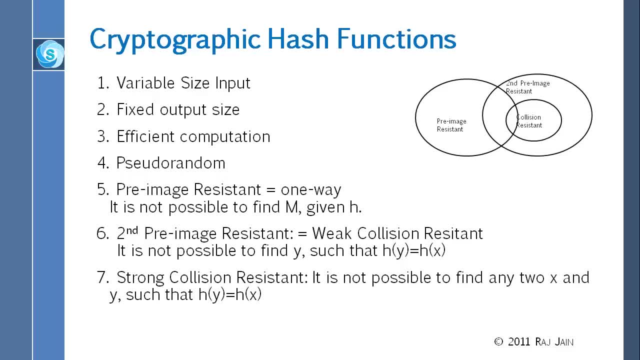 And the third one is strong collision resistant. So this is called weak collision resistant, the previous one. There are two names for it: Weak collision resistant or second pre-image resistant And the strong collision resistant. it is not possible to find any two, X and Y. 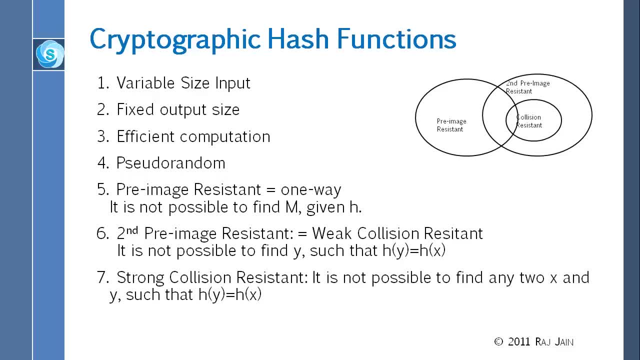 So it's not that I give you an H and you are trying to find out a Y Here. you just can go through the whole search and find any two X and Y such that they collide. You cannot find that. That is a strong collision resistance. 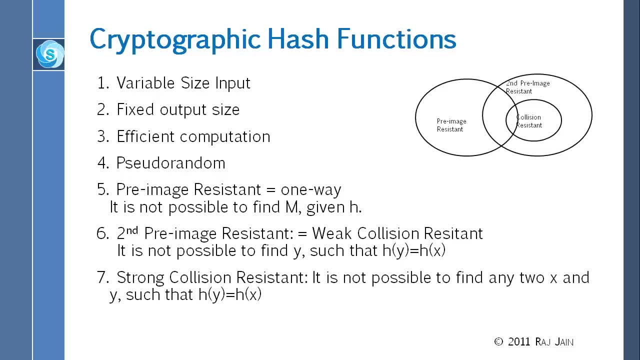 All right. And if you were to look into the Venn diagram, everything that is collision resistant obviously is second pre-image resistant as well, Because if you cannot find any two X and Ys, then you cannot find. given an X, you cannot find a Y. 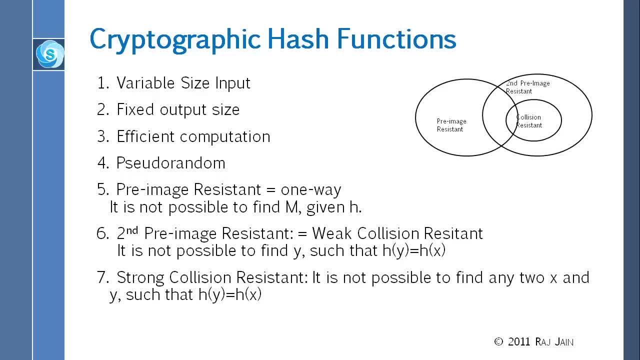 And some of the things which are pre-image resistant, maybe second pre-image resistant and some may not be. So this is not a proper subset like that, right? So the Venn diagram shows you that there are some hashes which will pass test 5 but will not pass test 6.. 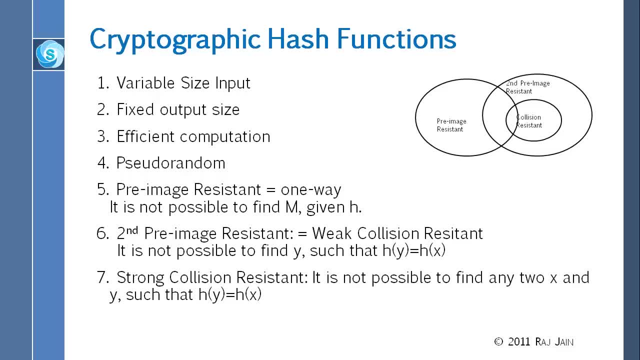 There are some that will pass test 6 but will not pass test 7.. The homework today is to basically verify that if the hash given hash passes all these seven tests- and the first four are trivial, there is nothing much to do there. 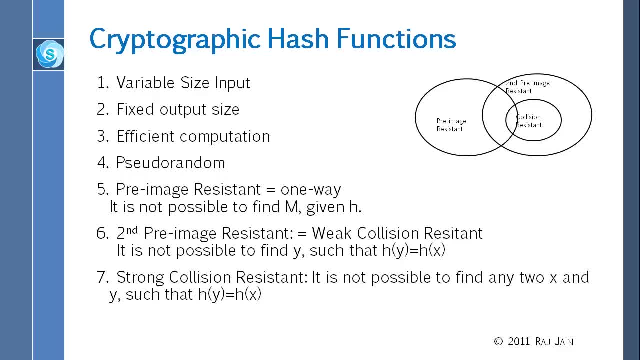 The three are basically: if you can find a counterexample that given H you can find M, or given X you can find Y, or given you can find two Xs and Ys, then it is not good for cryptographic hash. The impossible here simply means that it takes five years. 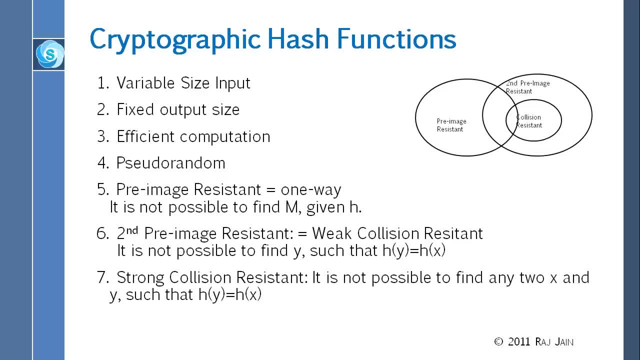 It doesn't mean you can do it in infinite years, Infinite years, In infinite years you can do everything. So it should be right, It should say it is not easy. I mean you know, if you think, if you put the word easy, yeah, I mean you know it's not possible. 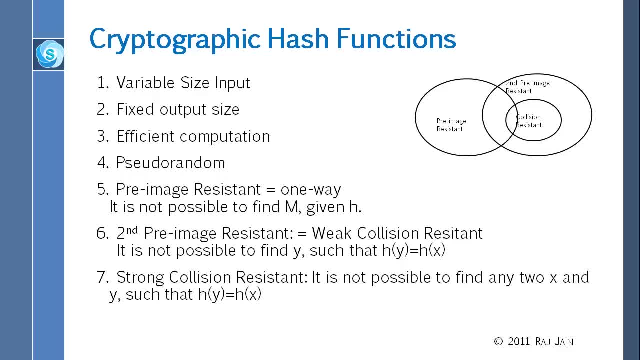 It means it is very difficult. It is that as the computing power increases, some things are resistant, So actually. so here is the thing I mean. that's a good point is that these boundaries are changing right. The boundaries of the hash functions are shrinking. 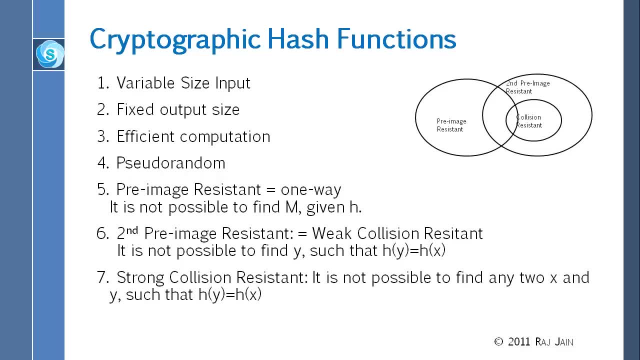 Previously there were lots of hash functions that would be called pre-image resistant, because they just required 2 raised to 32 computation, And now 2 raised to 32 can be easily broken. So they are outside this graph, outside this circle. It is very difficult. 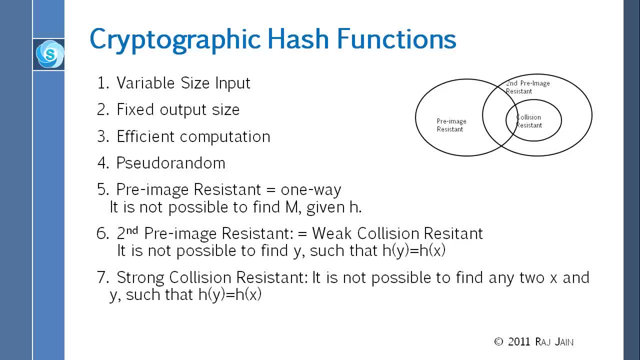 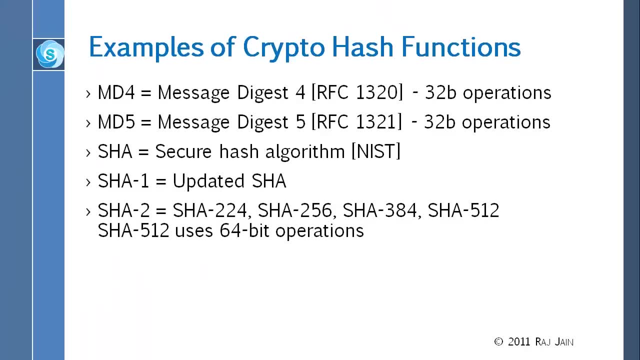 I should probably change that to say that it is very difficult to find M, It is very difficult to find Y, It is very difficult to find any two X and Y. All right, So the hash functions. So hash functions started with our friend Ron Revest starting MD2.. 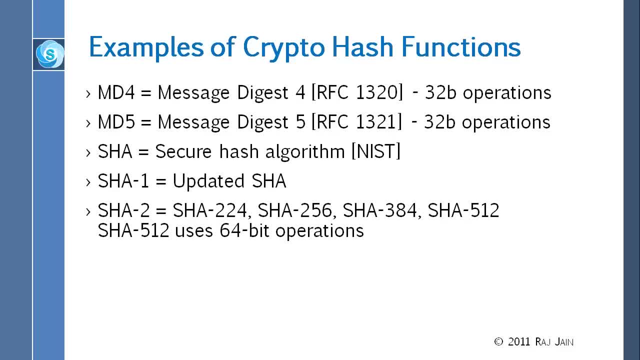 MD3., MD4., MD5. And after MD5, basically NIST took. I mean, basically MD5 was broken and NIST basically made a modification of MD5, made it stronger, called SHA. So SHA is the secure hash algorithm and then that was broken. 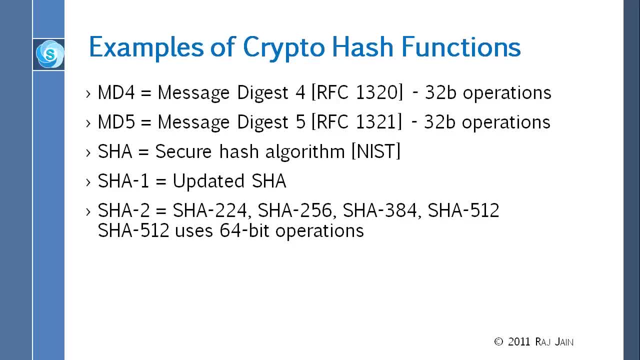 So then we have SHA1. And now that is easy to break- SHA2 and then SHA3. in the works, MD4 is described in RFCs and MD5 is described in RFCs. So this is all work being done in IETF. 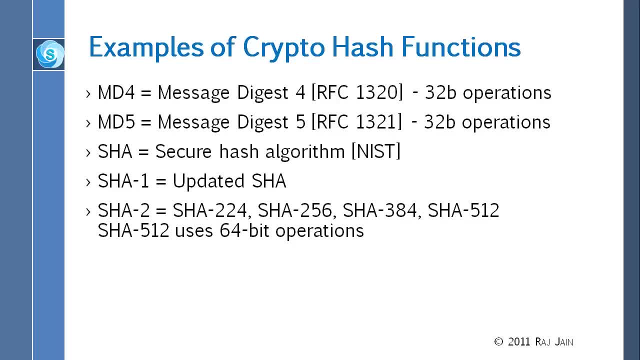 And then NIST took over from here And obviously these are designed for software, And so this is 32-bit, This is 32-bit, And these are going up higher And they are going up to 64.. 64-bit. 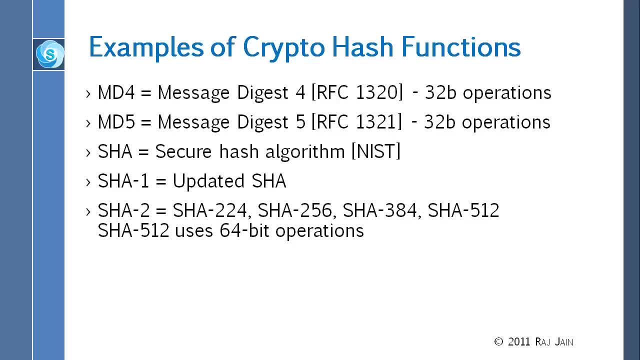 So anyway. So these are just in a sequence, basically building one on the other over the other. We will not talk about MD4 and MD5 here in this class much, except when they are starting with SHA. by the way. Now MD5, you have all seen. 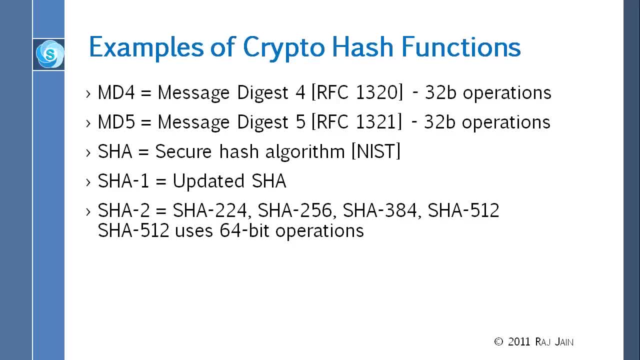 If you have downloaded any torrent or anything like that. they use MD5 hash And that's how we distinguish one file in the world from another file. If two files have the same hash, then torrents exist And torrent system cannot distinguish them. 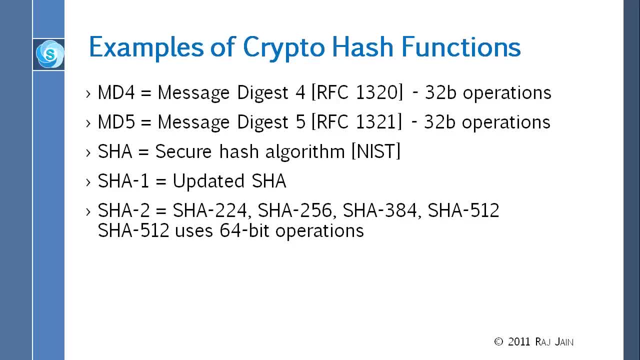 That's a cryptographic hash, So you cannot modify a file and then put it under the same torrent, because the torrent system will know that this is a different file. All right, So have you seen MD5 hash? Have you heard of it right? 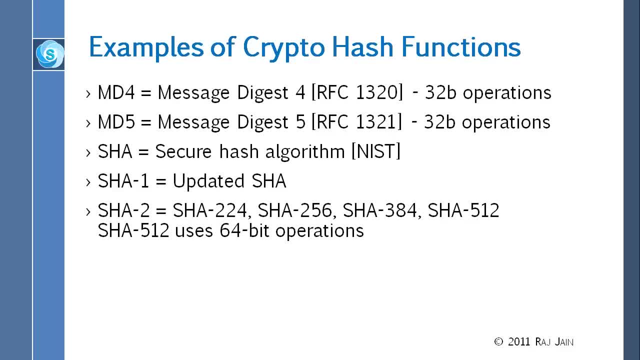 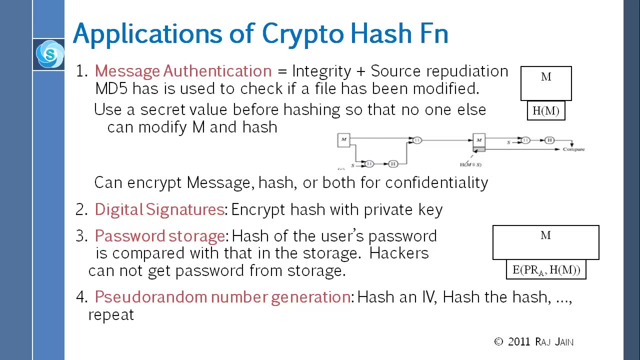 So that's now broken And so that means I mean you can break torrent, You can play games with that. That's another one, But basically, So the idea will be to start with SHA. Before we go to SHA, there are some applications as to why we need it, you know. 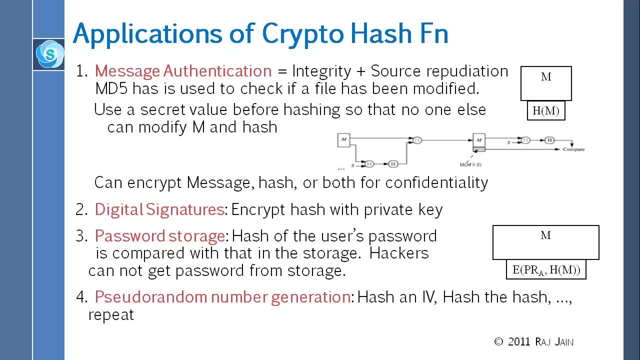 And then we go into hash, SHA, right. So first thing you need hash function is for authentication, And authentication means two things actually: Integrity plus source authentication. Actually, I should modify that All right, As shown in this picture here, actually it does not do the source modification. 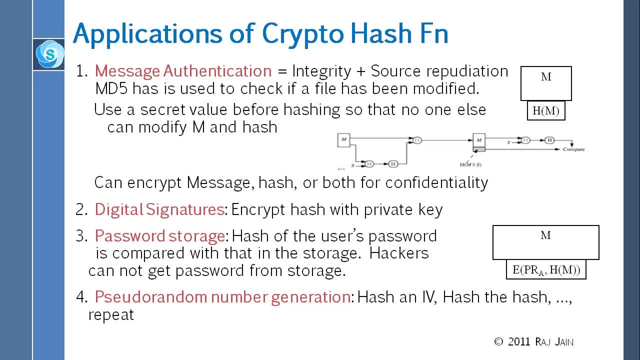 So this is a weaker definition of message authentication. We have a stronger definition, which is coming up in the next chapter, where integrity plus really the message authentication has to do with integrity plus source authentication. So you can verify two things. So here we'll just use the integrity part. 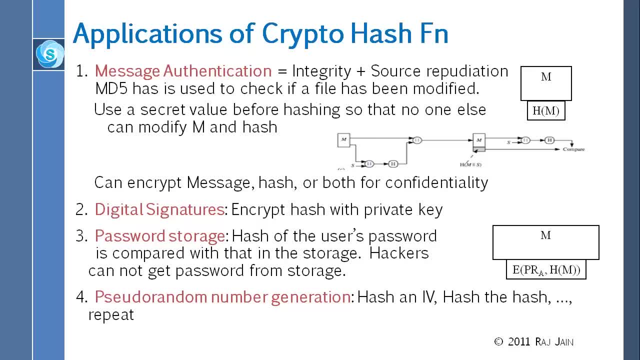 Although they call it message authentication, I would have called it message integrity- Is that we want to verify that nobody has modified it, And MD5 is used for that, And all we do is we take the original message and then we put the hash value. 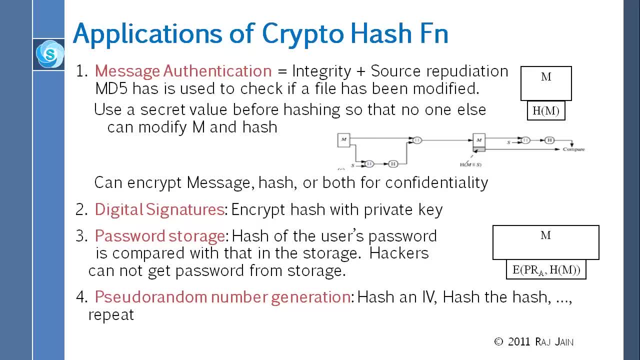 And so if you want to do source authentication, then you will have a secret value and then hash using that secret value So that nobody else can find that hash. So when somebody- only people who know the secret value- would have created that hash, 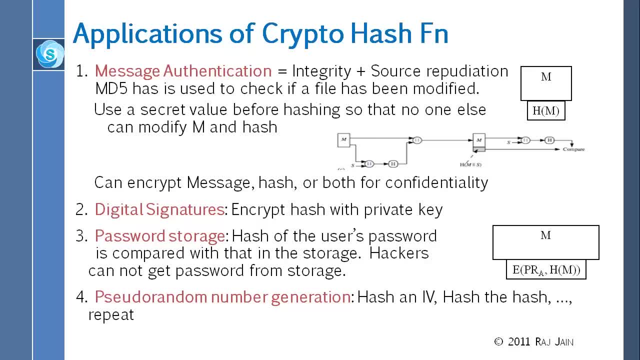 And therefore you can verify that. okay, you knew the secret and I knew the secret, So nobody else can make this message up, So source cannot deny, basically. So that's the kind of thing that you do: message authentication, And so you take a message, take a secret. 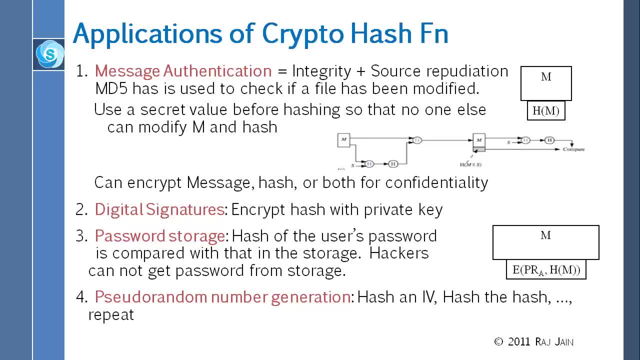 And these two lines in parallel means concatenate. Concatenate means you put one behind the other And then you run the hash. H is the hash, And whatever hash comes out, you concatenate with the message itself and you send it out. So basically, you have the message and the hash. 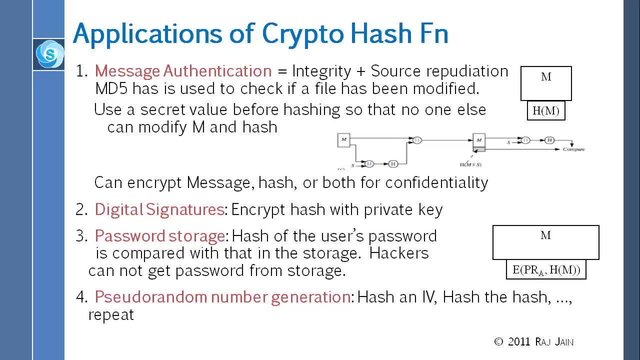 Send it out. The receiver can do the same thing. It can take the message and the secret and calculate the hash and compare with the hash that was sent, And that's what we do actually. So when you download an entire file, they come up with SFV. 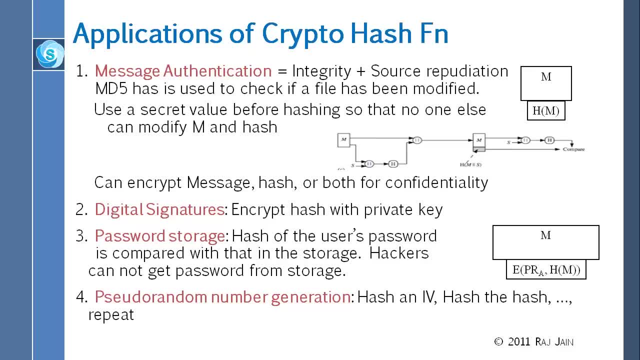 I think SFV stands for value or whatever. SFC, SFC is SFC, SFB- Anybody remember? There is a program that you run to verify that none of the files have been changed. You get when you get raw files or GIF files or something like that, you know, in 15 pieces or 32 pieces. 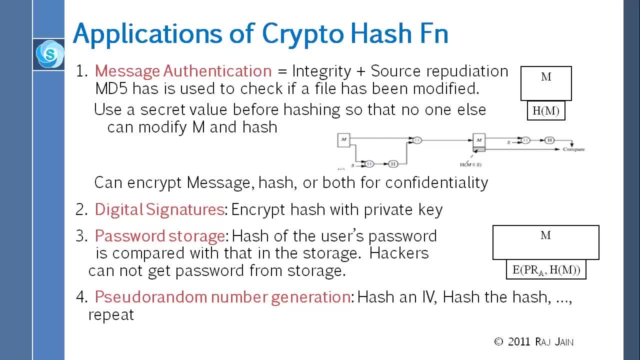 Then you want to make sure that all those files are in. nothing has been corrupted- Actually, nobody will modify them, but they get corrupted on transmission And so they're already set up. They send you a whole set of MD5 values for each file. MD5 value: 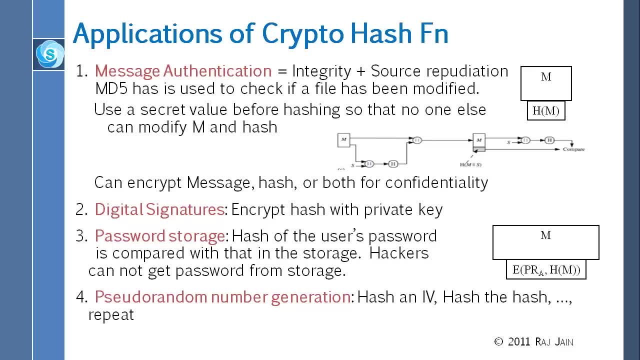 And you can calculate it very fast and check it out that the files are all perfect before you un-raw it or un-GIF it or un-next, whatever you want to do it right. So that is message authentication, which could be simply the integrated basically issue. 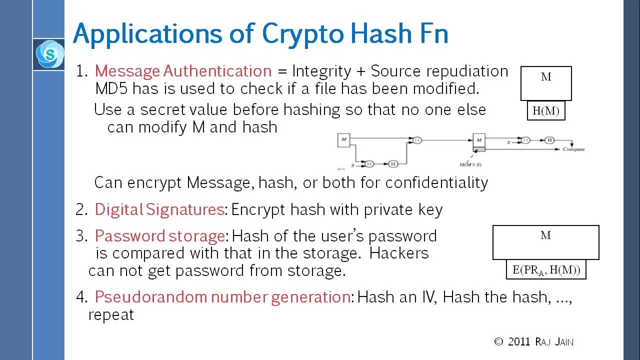 And then you don't need any secret value, because anybody can hash it and anybody can check it out, that the file is not modified. If you use the secret value, then it becomes real message authentication. The second thing is digital signature, which is almost similar to what we talked about, is that you hash it with a private key. 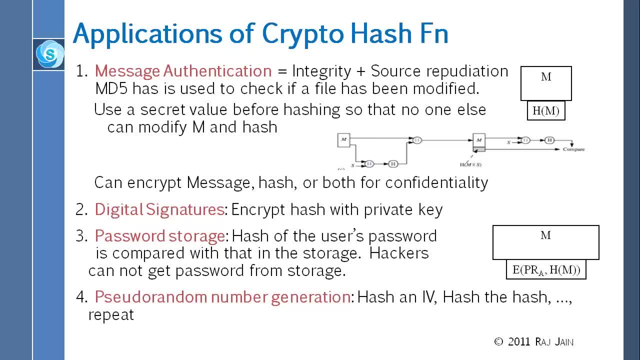 Then anybody can verify with the public key that it was you who hashed it And therefore we can put it into the court of the law. And so that's that one Password storage, So your password when it is stored on the computer. even the system manager does not know your password. 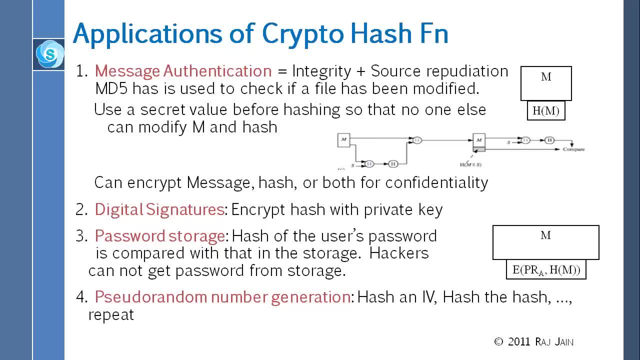 How is that possible? Because your password is not stored on the system. What is stored is the hash. Given the hash, the system manager cannot un-hash it to find out your real password. All right, And when you enter a password- username and password- it is again hashed and checked. 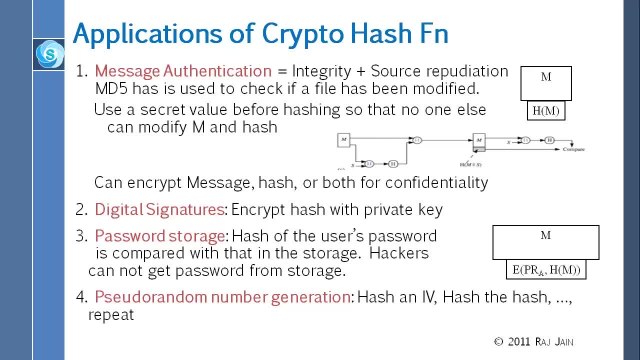 With the hash value. So the only hash values are used in the password And John the Ripper that the program you ran what that was doing was really trying out all possible hashes. So basically it was taking all the values, the ranges that you did, hashing it and comparing it with the value there that you were trying to un-hash.